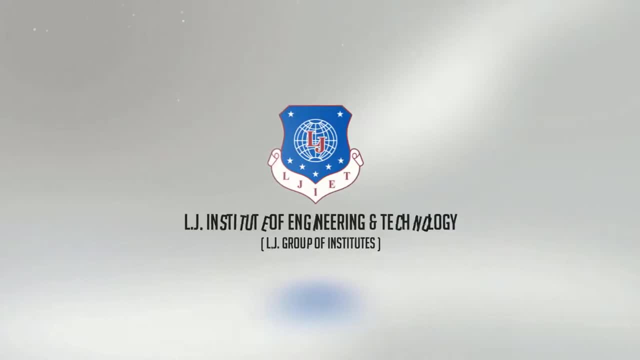 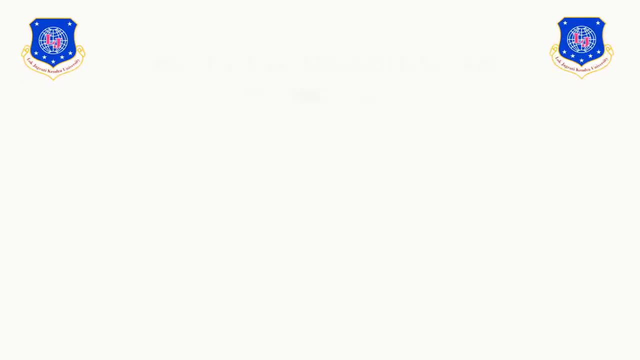 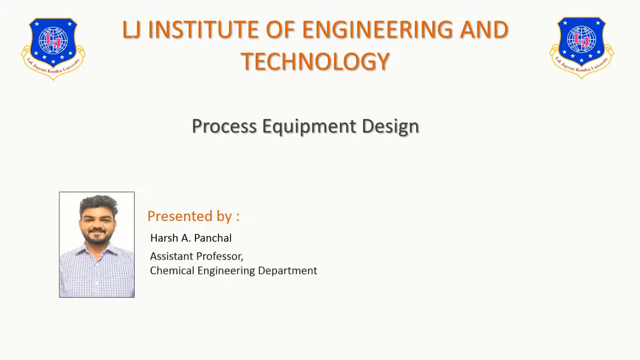 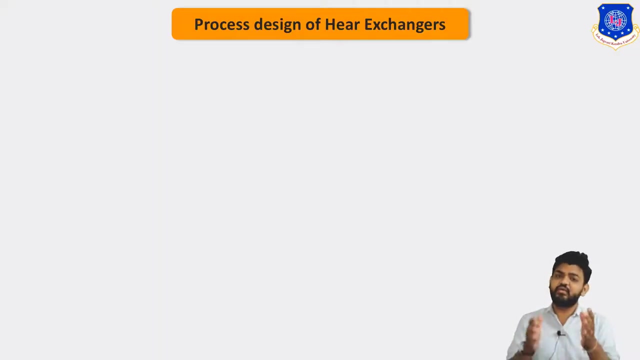 Hey guys, welcome to this video lecture series on the subject of process equipment design. I am Harsh Panchal, Assistant Professor in Chemical Engineering Department of LJ Institute of Engineering and Technology. Well, in a previous video of process designing of heat exchanger, we have understand different advantages and disadvantages of heat exchangers. 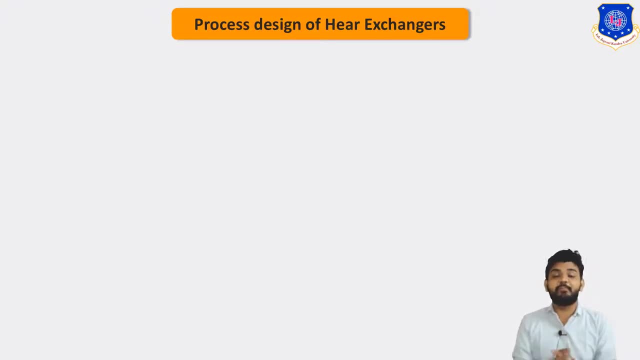 In which we have seen the U-tube type of heat exchanger, Then we have compared it with floating head type of heat exchanger. And lastly, we have also understand different advantages and disadvantages of fixed tube heat exchangers. And lastly, we have also understand how do we can allocate fluid, either hot fluid or cold fluid, through the shell side or through the tube side right. 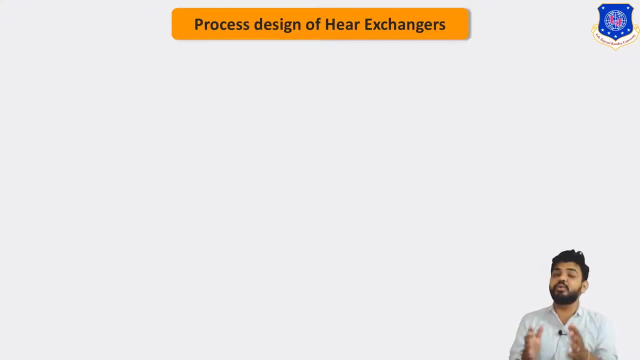 So all this theory part is again very important for the university exam. Now, after understanding all the theory part of this process- designing of shell and tube heat exchanger- we are going to understand how do we can actually design one heat exchanger. 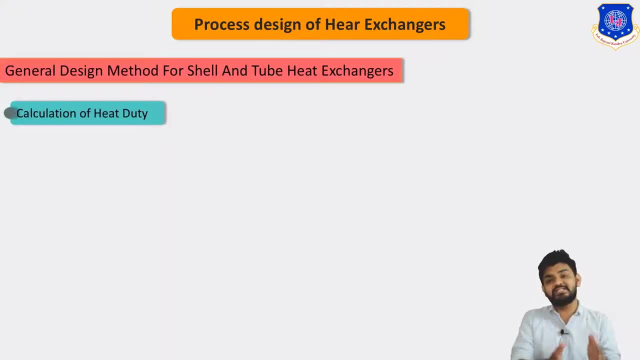 So let us just understand what are the general designing methods for shell and tube heat exchangers. Well, we need to follow certain steps in order to design one heat exchanger. So this step we are going to understand in this video, one by one, right? 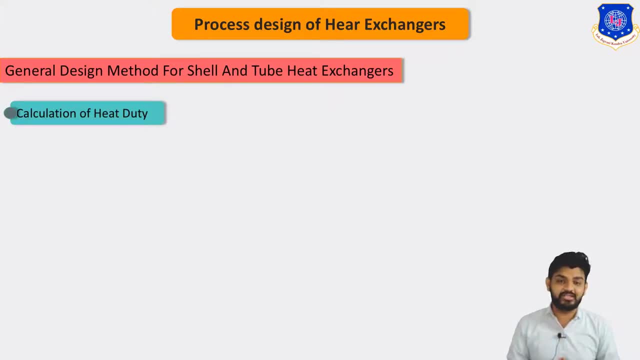 So the first and by far the most important step is heat exchanger. So the first and by far the most important step is heat exchanger. So the first and by far the most important step is heat exchanger. So the first and by far the most important step is to calculate heat duty. So, as you can see here, heat duty can be easily calculated by the most simplest equation for the heat that we have understand in a thermodynamic right. So, as you can see here, heat duty can be easily calculated by the most simplest equation for the heat that we have understand in a thermodynamic right. So, as you can see here, heat duty can be easily calculated by the most simplest equation for the heat that we have understand in a thermodynamic right. So, as you can see here, heat duty can be easily calculated by the most simplest equation for the heat that we have understand in a thermodynamic right. 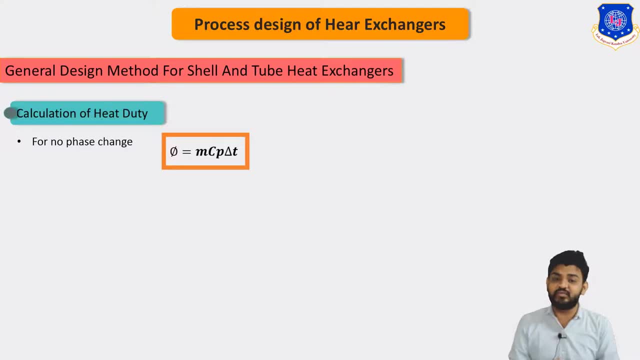 So, as you can see here, heat duty can be easily calculated by the most simplest equation for the heat that we have understand in a thermodynamic right, by the most simplest equation for the heat that we have understand in a thermodynamic right. 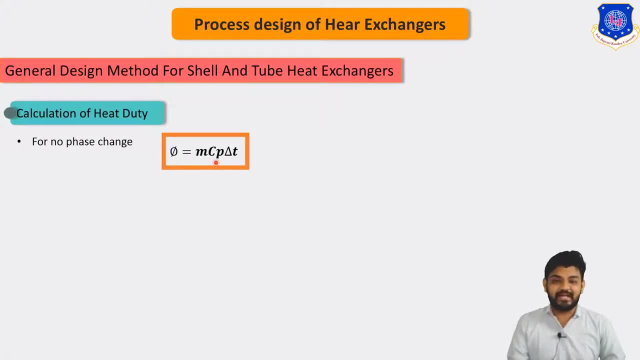 So that equation Q is equal to m, C, p, delta, t. right? we have also understand this equation in thermodynamics: 1. So for no phase change, that means when: whenever there is a no phase change in our heat exchanger, then we need to use this equation, that is phi. that is nothing but your. 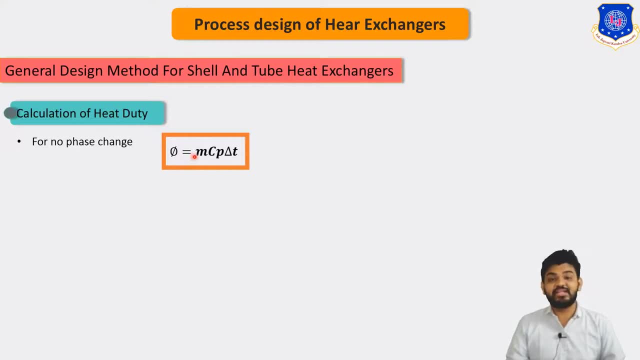 heat duty in kilowatt is equal to m, that is your mass flow rate. C, p is the specific heat of liquid into delta, t, that is inlet and outlet temperature of that particular fluid. Now, but what if the case is with the condensation right? that means there is a phase change. So in order to calculate, 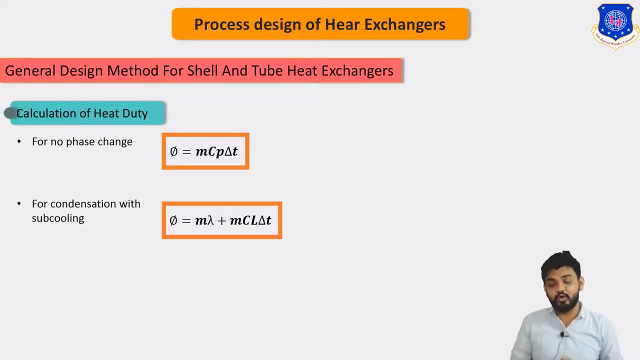 heat duty for a condensation plus sub cooling, then we have to use this particular equation, that is: phi is equal to m lambda, that is nothing But your latent heat plus C, m, that is mass flow rate of liquid. that is sub cooling into C l, into 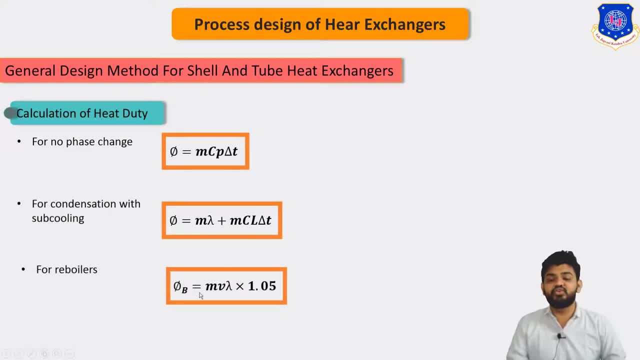 delta t right. and for the reboiler case we can use this equation, that is, phi b is equal to m into lambda multiplied by 1.05 right. So by using this three equation, we can calculate heat duty of our heat exchanger. and that is the first step in order to design heat exchanger. Now, after calculating, 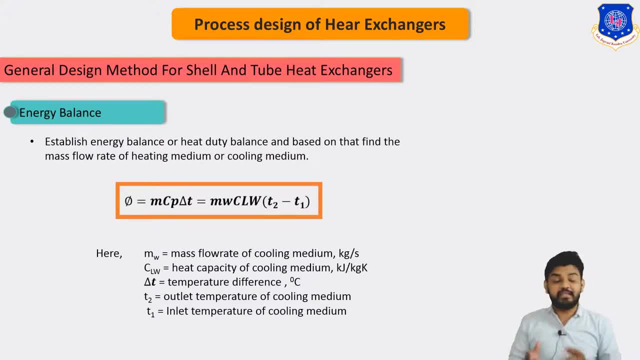 this heat duty. The second step is to calculate the mass flow rate of the secondary medium right secondary fluid. So for that we are using this energy balance equation because ultimately heat gain by cold fluid will be equal to heat lost by hot fluid right. So we are going to use that particular. 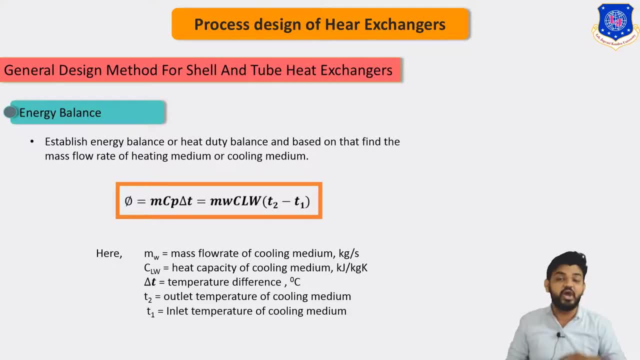 energy balance equation and we will calculate mass flow rate of secondary fluid right. So that can be done, as we have already calculated phi, that is m, C, p, delta, t, And then we need to compare it with m- w. that is mass flow rate of secondary fluid that we need to calculate into C l, into 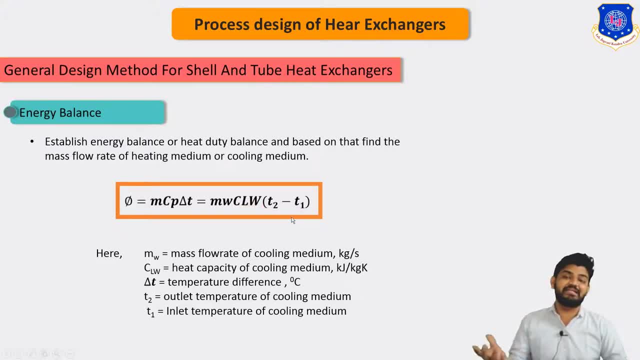 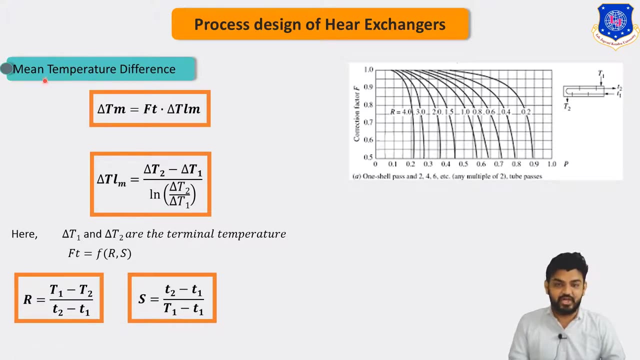 w in bracket T 2 minus T 1, that is inlet and outlet temperature of secondary fluid, right? So by doing this energy balance, we can easily calculate mass flow rate of secondary fluid. Now, after calculating this, our third step is to calculate mean temperature difference. right? so this particular mean temperature difference is: 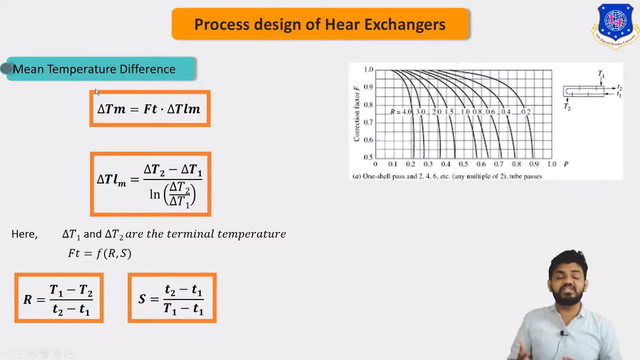 again very important and sometimes MCQ type equation can only be asked to calculate L and Td, that is logarithmic, mean temperature difference, right, or we can say mean temperature difference In a heat exchanger. we have two arrangement. The first one is the cross current right. So 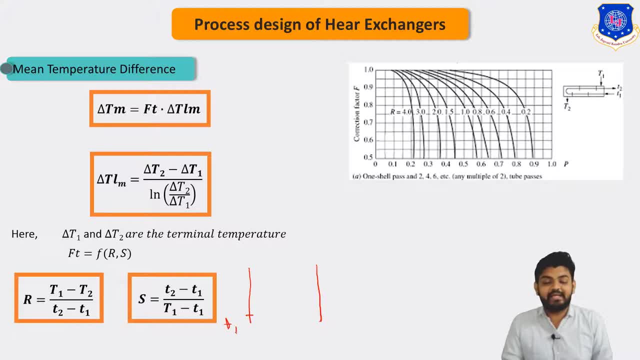 let us just suppose our cold fluid entering at T1 temperature and it get discharged at T2 temperature like this right, and it flows in this particular direction, Since we are using cross current or we can say countercurrent manner, So our hot fluid will enter from this side. that. 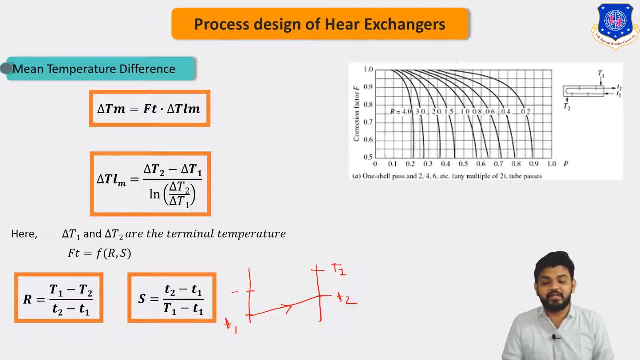 is with capital T1 temperature and it will exit at this particular temperature of T2, right? So you can see here, this is the, this is the manner, or we can say this is the countercurrent operation. This is the countercurrent operation of heat duty. So this particular difference will 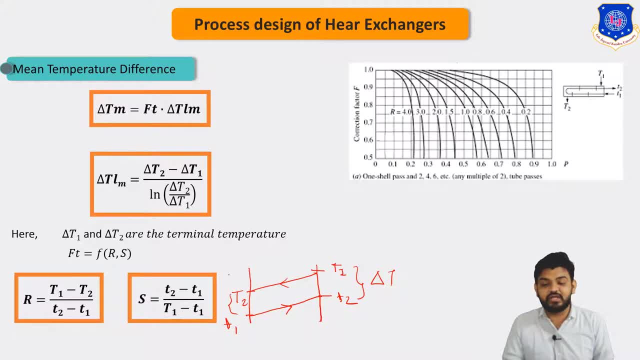 be called as delta T1, and this particular temperature difference we will call as delta T2, right? So now, using this T1 and delta T1 and delta T2 temperature, we need to calculate this LMT, right? So delta TLM, delta TM is equal to FT- into delta TLM. Now delta TLM can be calculated. 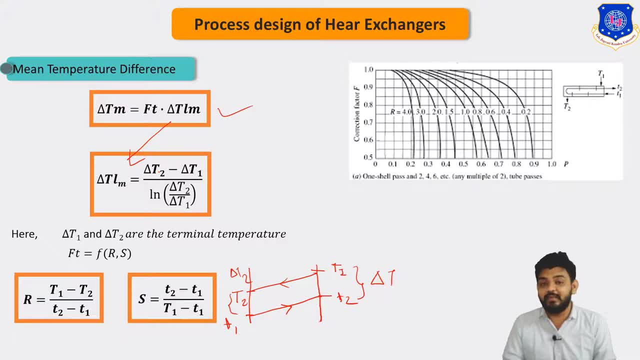 by using this formula, that is nothing but your logarithmic mean temperature, that is, delta T2 minus delta T1 divided by ln of delta T2 divided by delta T1,. right Now, if we replace this thing here and we need to calculate this value of FT, well, this value of FT is nothing but the correction. 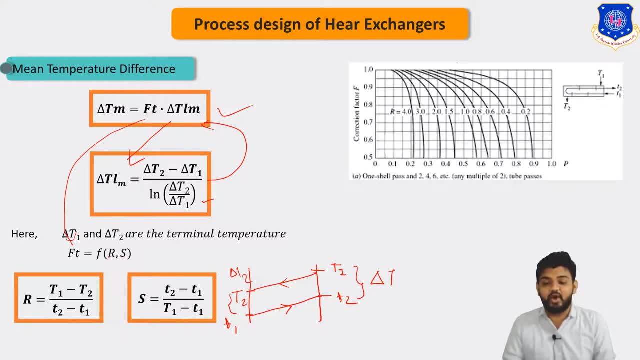 factor right Correction factor value greaterly depend on value of R and S. This R is nothing but temperature difference of hot fluid divided by temperature difference of cold fluid, and this S is nothing but temperature difference of cold fluid. So by using this R and S value we can easily calculate this correction factor FT. So FT is: 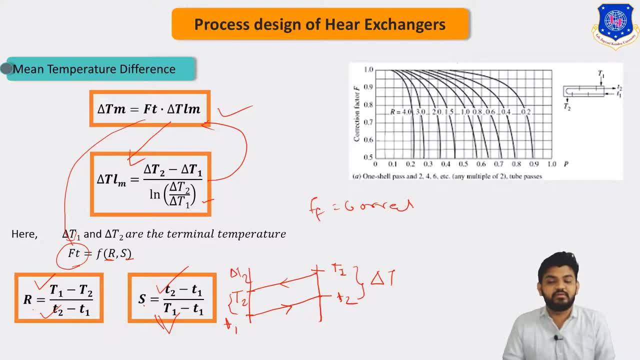 equal to nothing but your correction factor, right? So how do we can calculate this value of FT? As you can see here? we need to find first R value. You can see here in this particular graph, this is the R values, right? So we need to decide what is the R value. Let us suppose our R value. 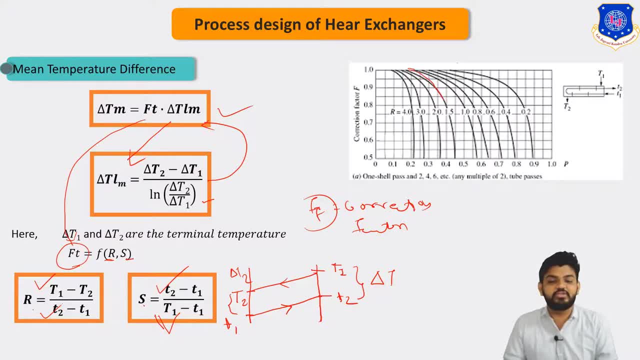 coming out to be 1.5.. Then we need to follow this particular graph right And now. after that we need to calculate value of S. On the X-axis we have value of S. Let us suppose our value of X is. 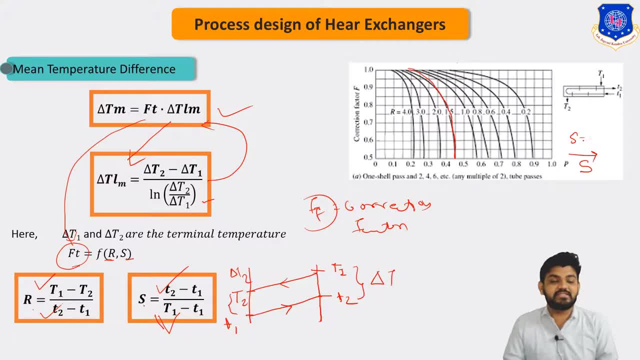 around 0.4, right. Let us suppose S is equal to 0.41.. So from here we will look at this: 0.41, right? So if we move this to S, then we will get 0.41.. So if we move this to S, then we will get. 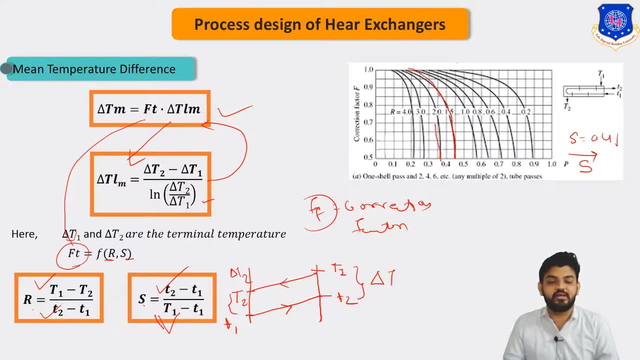 0.41, right. So from here we will look at: this is the 0.41, right. So if we move this to S, then we this two point. if we interchange this two point, you can see here like this: So ultimately it will: 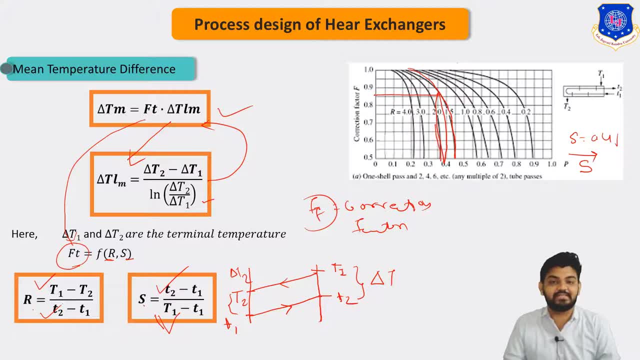 give us the value of F on the x axis, on the y axis right. So here from the graph, value of Ft is something around 0.86.. So this is how we can calculate value of Ft. that is your correction. 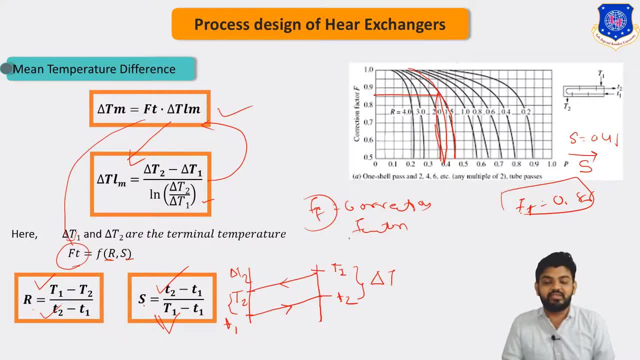 factor And value of Ft. here you can see that the value of Ft is equal to 1 for 1, 1 heat exchanger right 1, 1 heat exchanger. So by using these formulas we can calculate delta Tm. that is our. 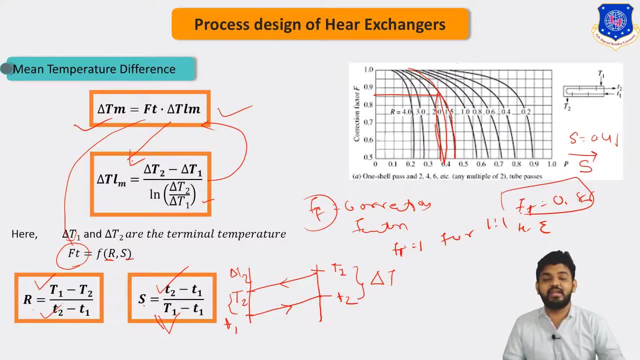 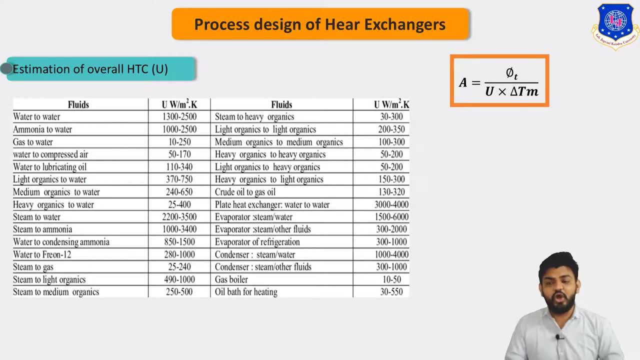 third step Now, after calculating this delta Tm, we need to assume the overall heat transfer coefficient in the case of challenging heat exchanger. So, in order to assume this capital U, we can use this particular table. as you can see here, we can use this particular table. 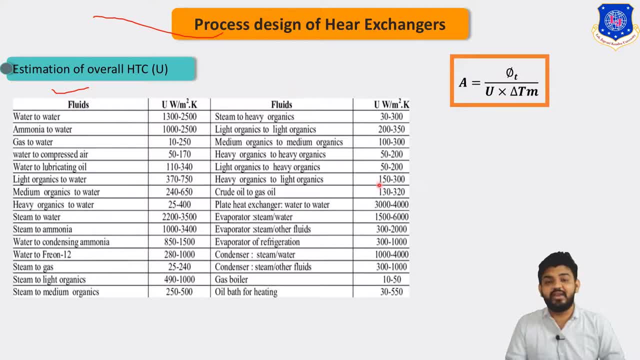 in which, for the different fluid, the values of capital U is given. Let us just suppose our fluid is water, then we can assume value of capital U between 13,000 to 25,000, right. In a similar way, if our fluid is crude oil, 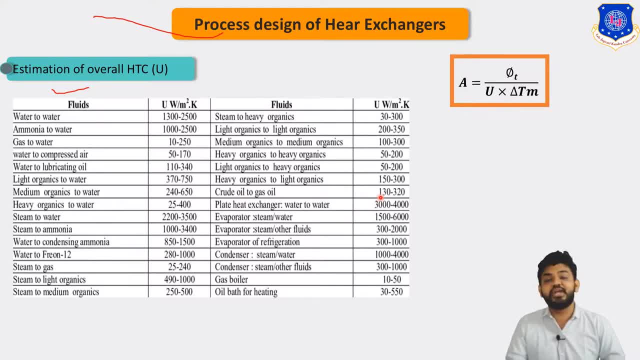 right. then we can assume U from 130 to 320.. So, based on this table, we can assume different value of capital U, right? And based on this capital U value, we need to calculate area provided. So, as you can see here, by using this particular formula we can calculate. 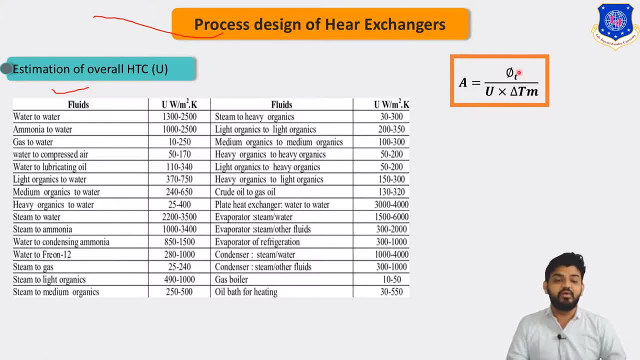 area provided as A is equal to phi. that we have calculated in the very first step- U we have already assumed, and in the third step we have calculated delta, Tm, right. So by using all this information we will calculate value of area provided. Now, after calculating, 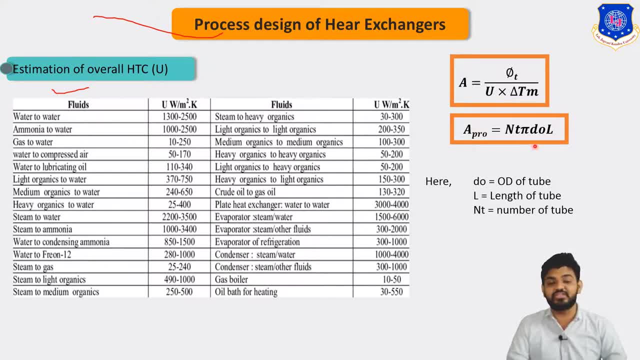 this area provided. we will compare this area provided with the equation of area provided equal to number of tubes into pipe, into outer diameter of tube, into length of tube right, that is, phi dL into number of tubes. So this will ultimately give us the value of NT right This outer. 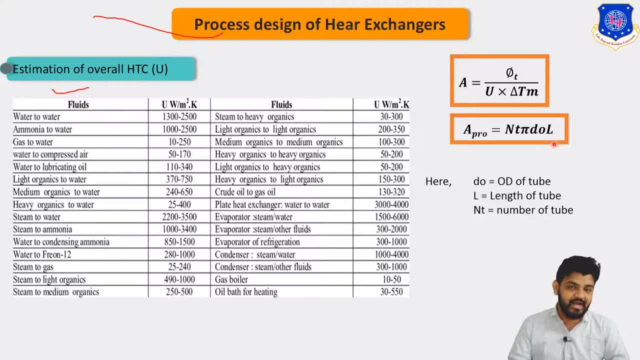 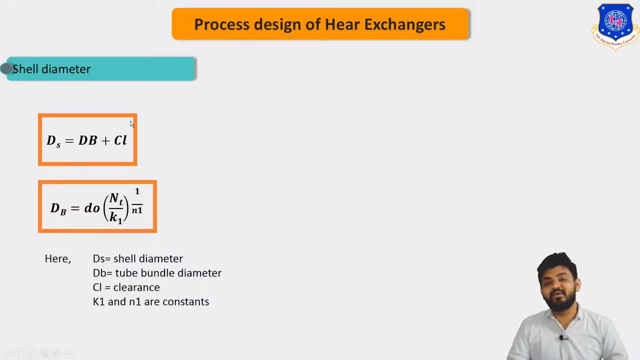 diameter of tube and length will be given to you in the example right. So after calculating NT, we need to calculate the value of shell diameter. That is our fifth step. You can see here in the shell diameter we can use this particular formula. This dS means the 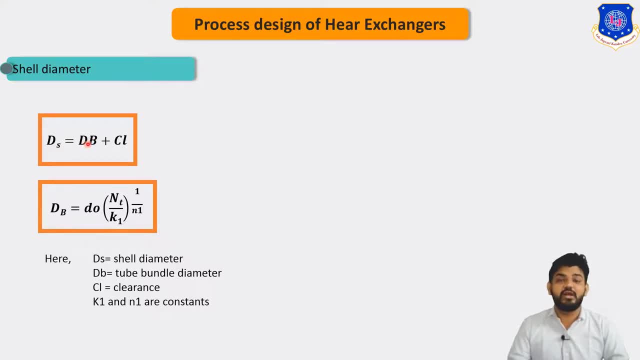 shell diameter is equal to dB. that is nothing but your bundle diameter, that is tube bundle diameter. as we have already understood In the previous lecture, we have one bundle of tube right? So in order to determine the shell diameter, we need to consider that bundle diameter as well. Bundle diameter plus. 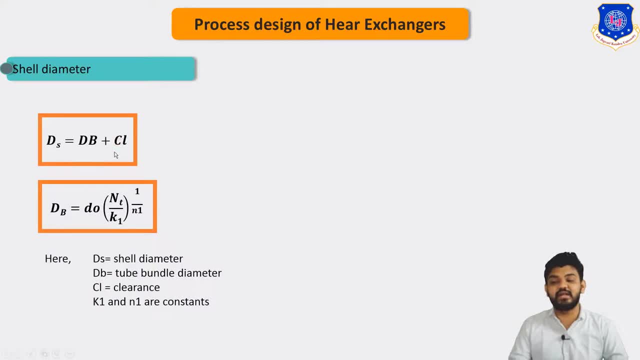 the clearance. right, we are going to add this clearance, as you can see here, And this clearance can be selected from 75 mm to 100 mm. right, But how do we can calculate this bundle diameter? Well, this bundle diameter can be easily calculated from this particular 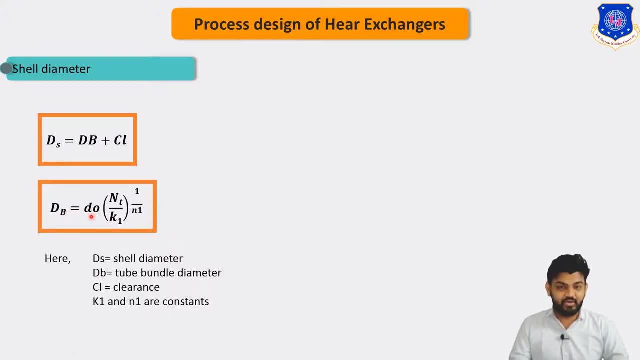 formula That is, dB is equal to outer diameter of tube. So this is the outer diameter of tube into number of tube divided by k1, raised to 1 minus 1 divided by n1.. Here k1 and n1 are the constant right. So value of k1 and n1 will be given to you in example itself. So 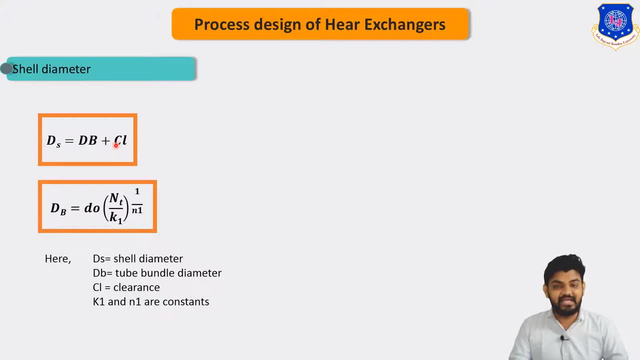 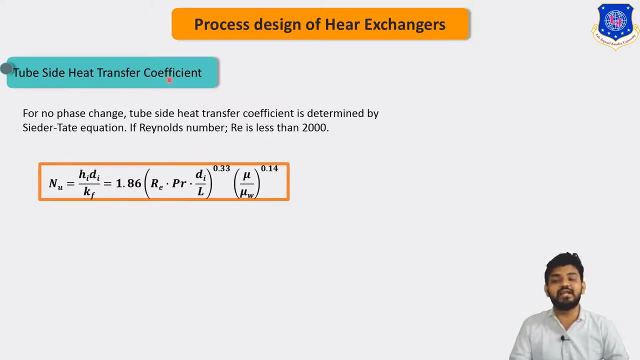 by. after calculating this diameter, we are going to add this clearance and we will ultimately get shell diameter. Now, after this fifth step, the sixth step is to calculate tube side heat transfer coefficient. Well, tube side heat transfer coefficient can be calculated with the help of different example. 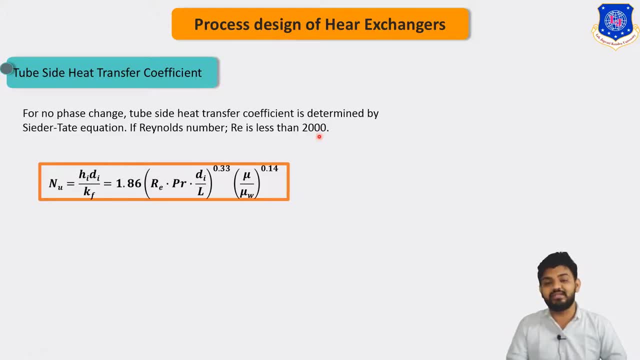 When our Reynolds number is less than 200, you can see here, the Reynolds number is less than 2000,. we can use this particular formula of Seder-Tate equation that we have understand in the fourth semester of heat transfer, right? You can see here, this is the third number. 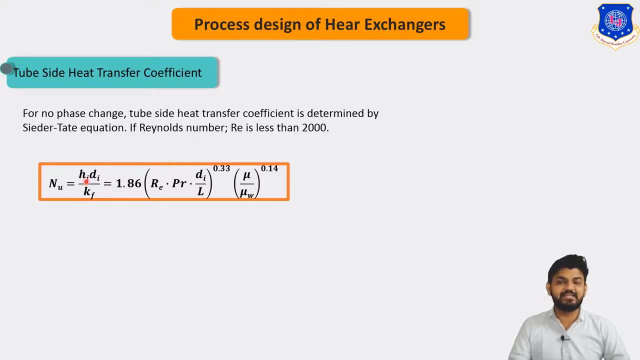 that is equal to h i, d i by k i h i means heat transfer coefficient on tube side, d i means tube side diameter and k f means tube side fluid thermal conductivity. that is equal to 1.86 into Reynolds number, Prandtl number, into d i inside diameter of tube divided by: 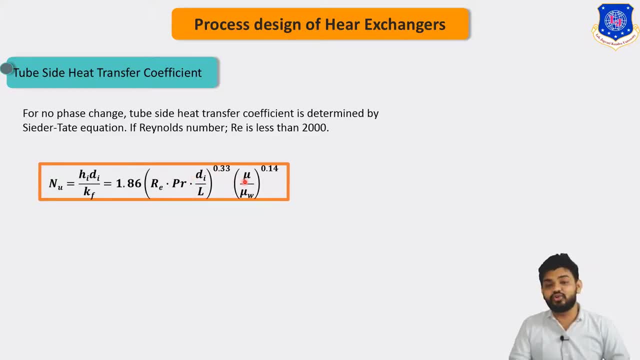 l, raised to 0.33, multiplied by viscosity of fluid. divided by viscosity of fluid near to the wall, raised to 0.14, right. In some cases, this value of u by uw is taken to be 1, right because the viscosity of fluid do not changes with respect to temperature at the wall. right. 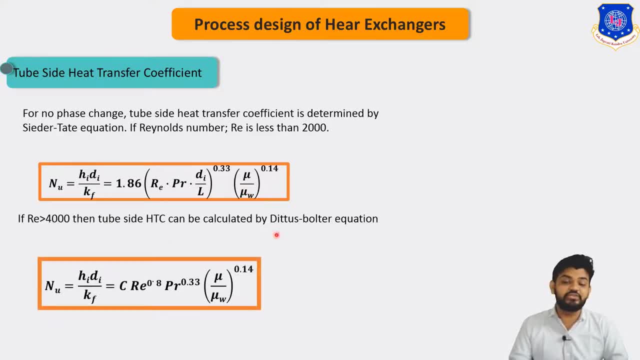 For the value of Reynolds number greater than 4000, we can write it as 0.14.. So this is 2000.. We can use this Seder-Tate equation in order to calculate heat transfer coefficient. that is equal to Nusselt number into C. that is nothing but your one constant into Reynolds. 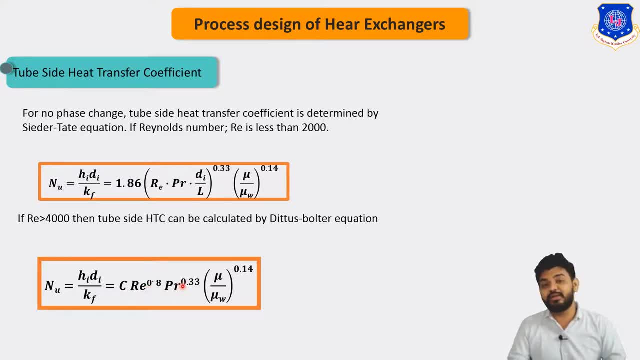 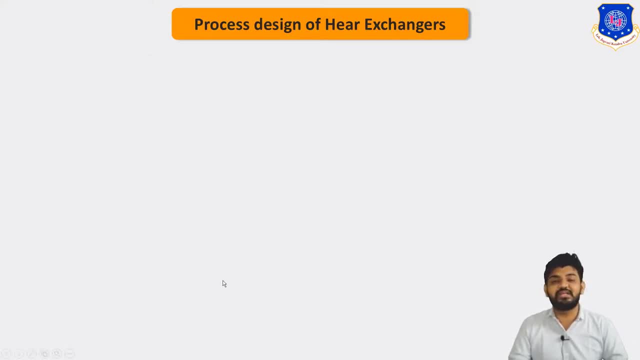 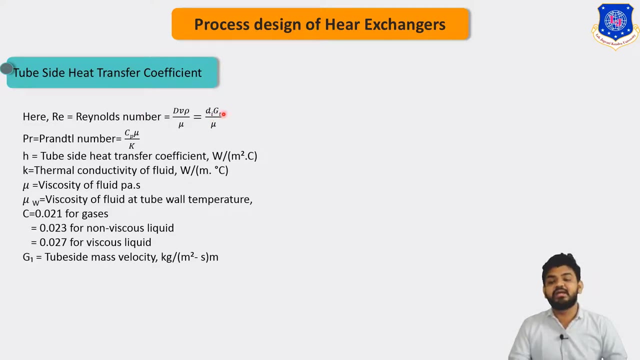 number raised to 0.8 into Prandtl, number raised to 0.33 into mu, by mu w raised to 0.14, right. So in this particular equation, value of C is need to be calculated. So, as you can see here, Reynolds number can be calculated by d V, rho, by mu or d i into. 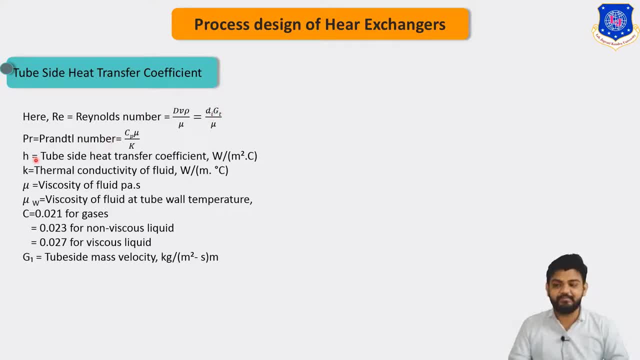 gt by mu, right, Then Prandtl number is cp. mu by k. hi is nothing but your tube side heat transfer coefficient, kf, that is fluid thermal conductivity. mu is equal to viscosity, mu w is viscosity at the wall of tube right, And value of c is equal to 0.021 for gases and it is equal to 0.023. 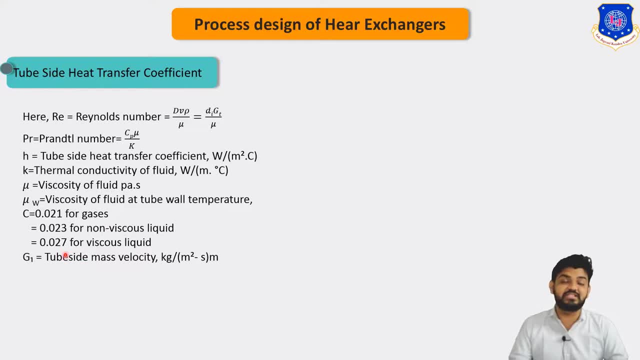 for non-viscous liquid and for the viscous liquid it is 0.027, right, And this gi is nothing but your tube side mass velocity. So now our task is to calculate this gi. as you can see here, gi can be calculated by mass flow rate divided by tube side flow area. So how do we can calculate? 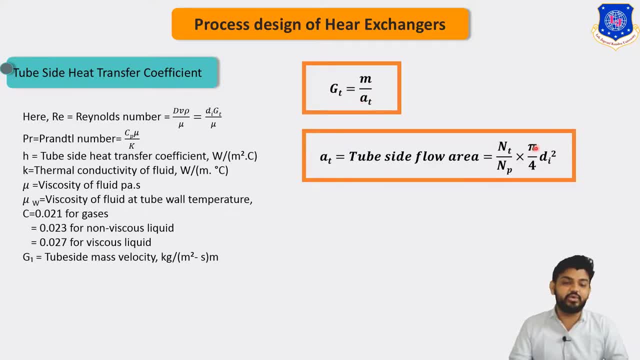 this tube side flow area, that is nothing but 80, is equal to pi by 4 d square. that multiplied by number of tube divided by number of passes, right? So we need to decide how much number of tube that we need to take and how much passes we have to provide. So after calculating this, 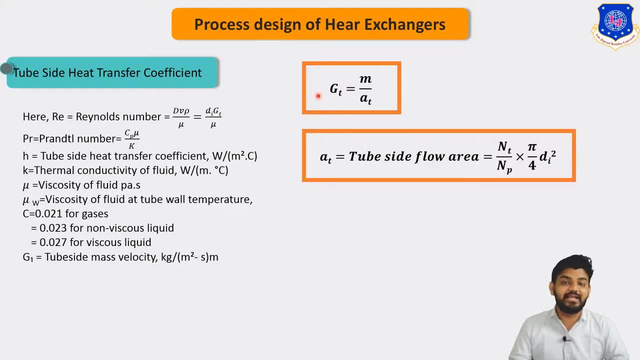 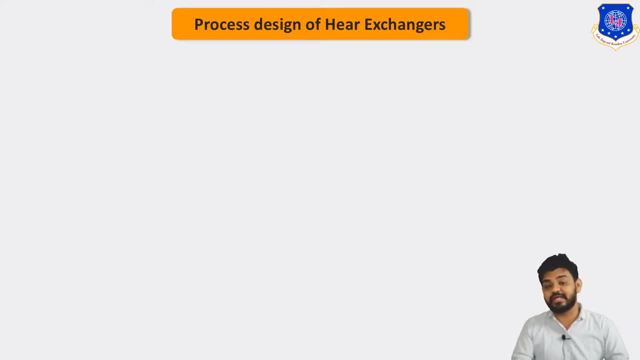 80. we will substitute inside the gt, then we will calculate the value of gt. based on that, we will calculate the value of Reynolds number and then, based on this Reynolds number, we will use either this Seder-Tate equation or the Deters-Beuters equation. right, So this was all about the heat. 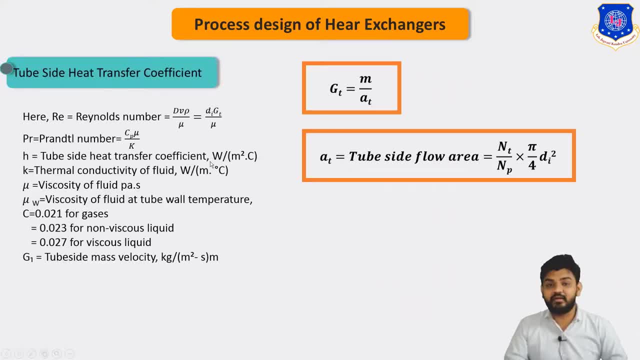 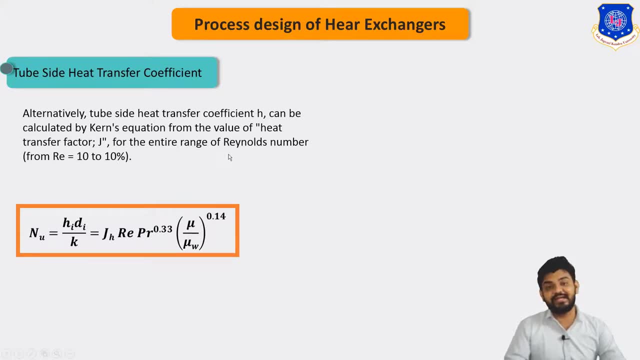 transfer coefficient: calculation for the tube side. right Now there is one more formula, that is generalized formula, in order to calculate the tube side heat transfer coefficient, and that is to jh into Reynolds number, into Prandtl's number, raise to 0.33, into mu by mu w, raise to 0.14.. 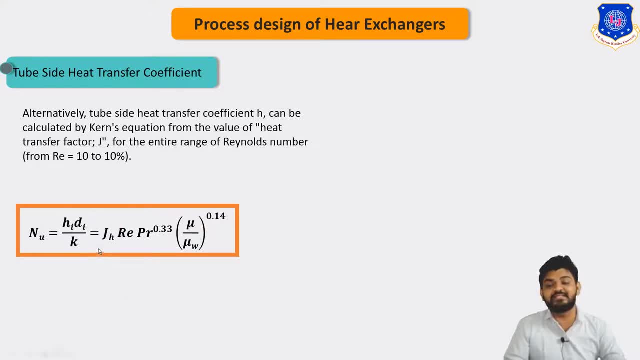 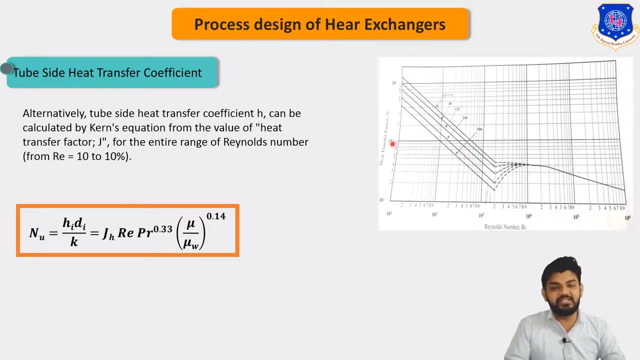 In this particular equation, the value of jf can easily be calculated from this particular graph right, Based on the value of Reynolds number. we can calculate this value of jh right And we have to replace this value of jh in this equation, So this particular equation can be used for any. 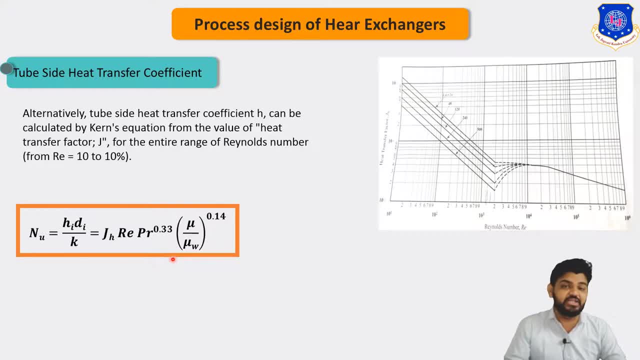 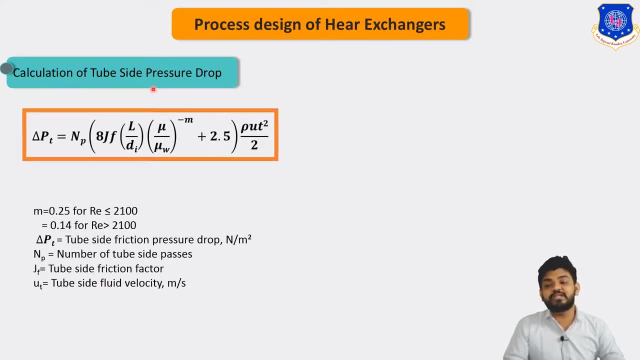 number of Reynolds right, So we can say that it is generalized equation. Now, after understanding this tube side heat transfer coefficient, the next task is to calculate the tube side pressure drop. So in the next step, we are going to calculate the tube side pressure drop by using this particular equation, that is, 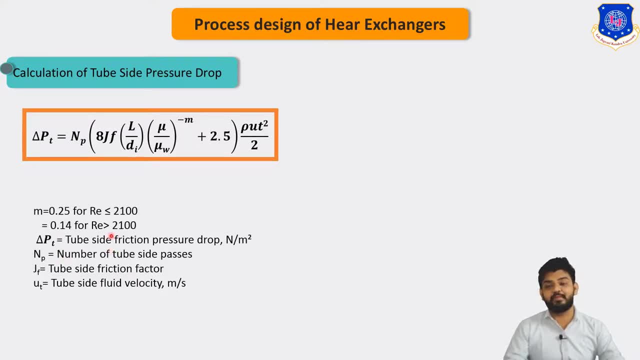 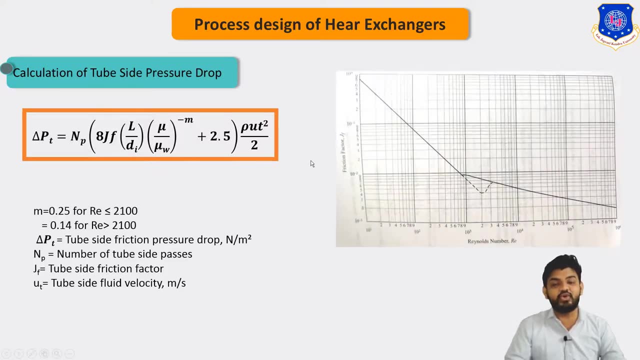 delta Pt is equal to tube side pressure. drop right Into NP, that is, number of pass into 8, into 8 jf. This jf can again be calculated from this particular graph, based on the Reynolds number right Into L divided by di into mu, by mu w, raise to minus m plus 2.5 rho into velocity, raise to 2,. 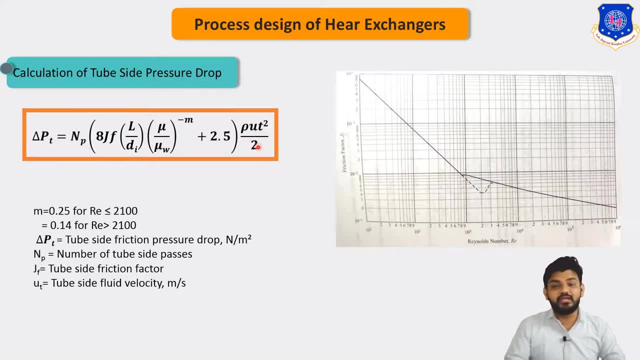 right. That is, ut raise to 2 divided by 2.. So this particular equation is being used in order to calculate the heat transfer or pressure drop through the tube side right. In this equation we are using this value of jf and that can be calculated from this particular graph. 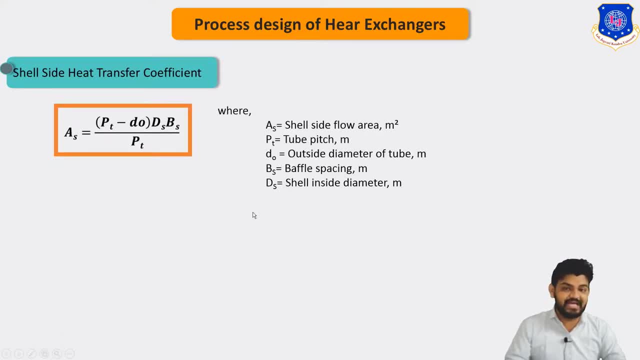 right Now, after calculating this pressure drop, our next task is to calculate the shell side heat transfer coefficient. Well, in order to calculate the shell side heat transfer coefficient, we have to follow certain procedure. In the very first step, we have to calculate this shell side flow. 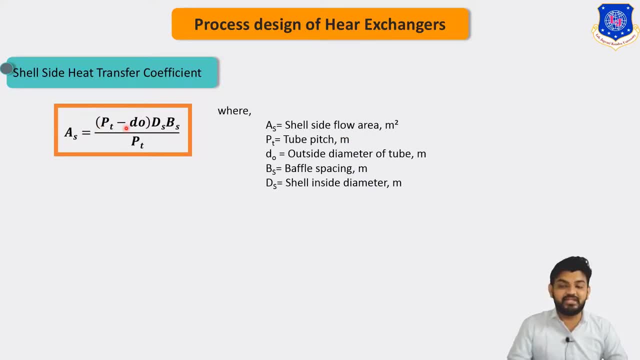 area that is equal to, As is equal to Pt minus Do. This Pt is nothing but your tube pitch. that we need to calculate, Then Do is outer diameter of tube into Ds, that is diameter of shell Into baffle spacing, that is Bs divided by Pt. Now we need to calculate based on this As value. 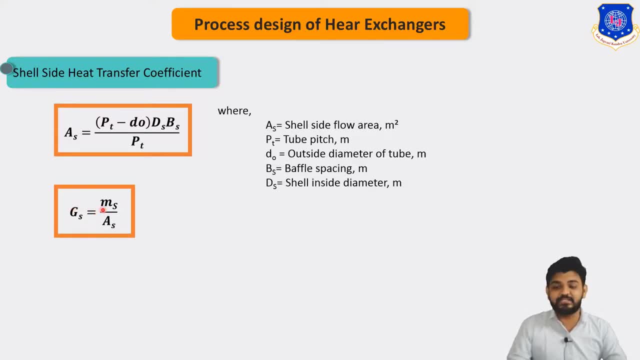 we need to calculate the shell side, mass velocity, that is, mass flow rate divided by area. Now, based on that, we are going to calculate the value of velocity that is Us is equal to mass flow rate divided by density. So, by using this formulas, we need to calculate three things, that is As: 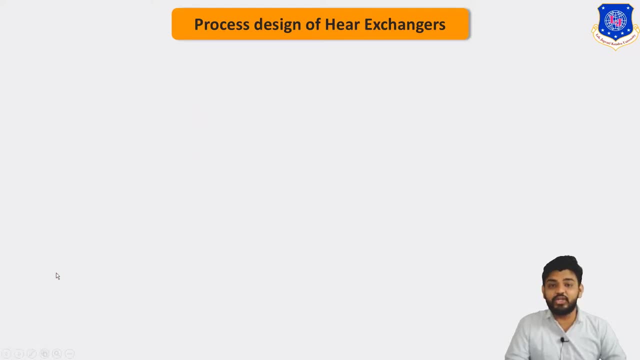 Gs and Us. Now, after calculating, we have to calculate equivalent diameter of the shell, and that can be calculated for the square pitch arrangement by De is equal to 1.27 divided by Do bracket Pt raised to 2. that is your pitch minus 0.785 into Do raised to 2.. So this particular equation is only applicable for the 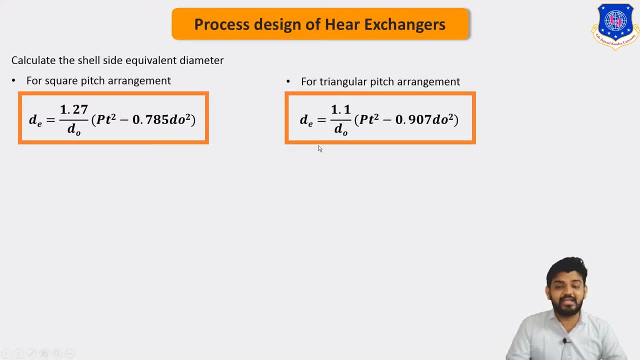 square pitch arrangement, And for the triangular pitch we can use this equation, that is: De is equal to 1.1 divided by Do into pitch square, minus 0.907 into DO square. This DO is outer diameter of the tubes right. So after calculating this equivalent diameter, the next task is to calculate shell side. 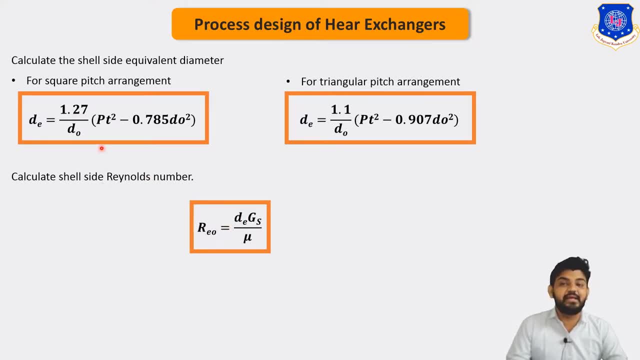 Reynolds number and that is equal to DE. that is equivalent diameter into mass flow rate divided by viscosity. After calculating Reynolds number, we need to calculate Prandtl's number for the shell side, that is Cp, mu by K. Now, after calculating all this information, we have to 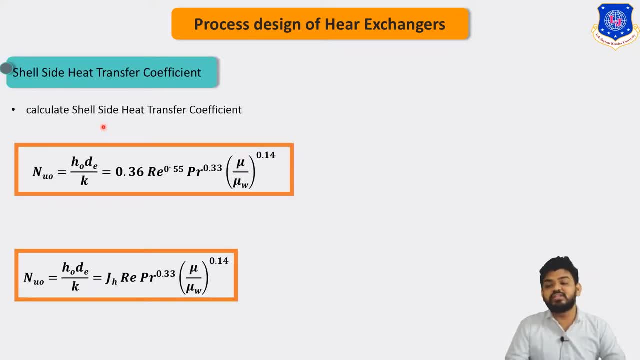 calculate shell side heat transfer coefficient using this particular equation. So that is: Nusselt number for the shell side is equal to HO, DE by K. that is heat transfer coefficient for shell side into this equivalent diameter multiplied by its, multiplied by thermal conductivity, which is equal to 0.36. Reynolds number raise to 0.55. Prandtl's number raise to 0.33 into mu by: 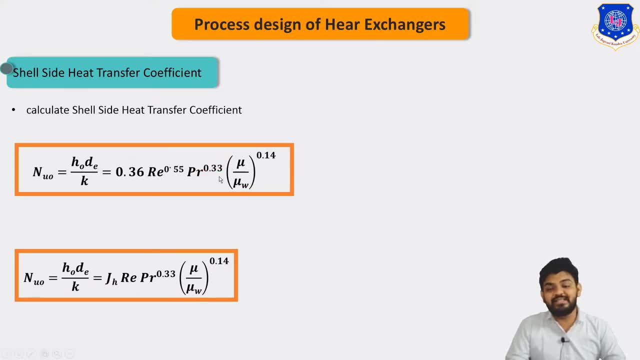 mu W raise to 1.0.14.. Now again, there is one more generalized formula in order to calculate heat transfer coefficient for the shell side, and that is equal to Nusselt number is equal to JH RE into PR raise to 0.33 divided by mu, by mu W raise to 0.14.. So by using this equation, we can calculate: 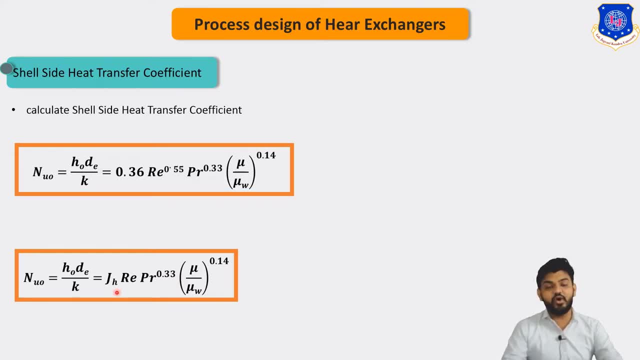 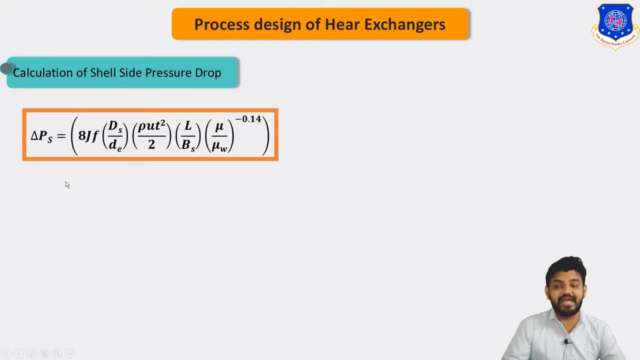 heat transfer coefficient based on shell side. Again, this value of JH can be easily calculated from the graph. Now, after calculating this shell side heat transfer coefficient, our next task is to calculate the shell side pressure, rho, And that can be calculated by this equation, that is, P, s is. 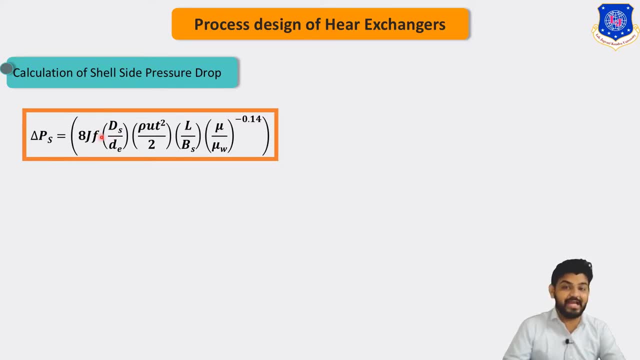 equal to 8, into JF Again. this JF value can be calculated from the graph right: Into d s, that is your diameter of shell divided by equivalent diameter. into rho ut square divided by 2.. This ut is again nothing but your velocity through the shell. into L divided by b s, that is baffle spacing. 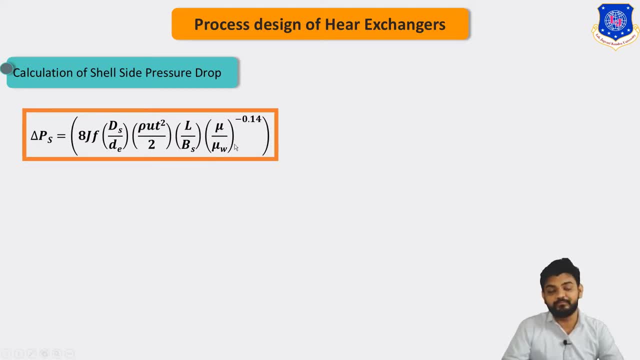 into mu by mu W raise to minus 0.25.. So you can see here all the information here. This P? s is nothing but the pressure drop. This d? e is equivalent diameter, L is length of tube, U, b, that is shell side velocity. Mu is. 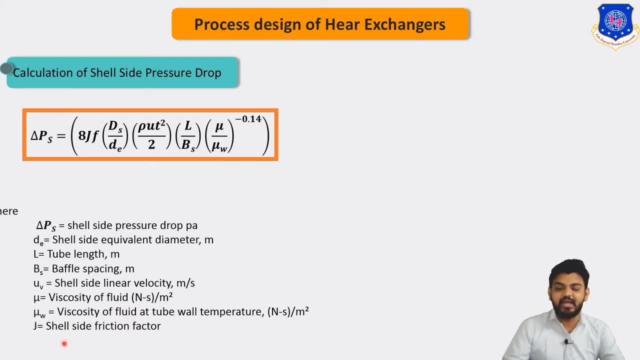 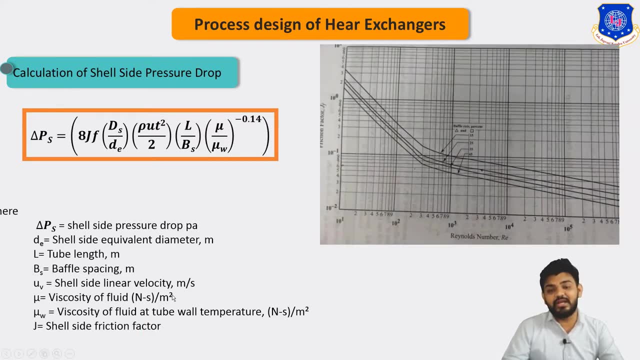 viscosity. Mu, W is equal to viscosity at the shell side And lastly, JH is the shell side friction factor. that can be calculated from the graph. So, after calculating that, that can be calculated from this particular graph, right? So after calculating this pressure drop, our next task is to calculate the overall heat transfer. 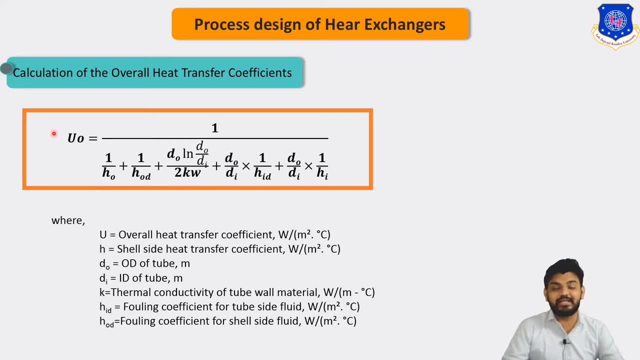 coefficient, While the overall heat transfer coefficient, U naught, can be calculated by this formula: that is equal to 1 divided by 1 upon HO plus 1 upon HOD. that is nothing but the fouling factor for the shell side right, Plus DO into ln of DO, divided by DI, divided by 2 into KW, that is. thermal conductivity. So this is the pressure drop. So, after calculating this pressure drop, our next task is to calculate the overall heat transfer coefficient. While the overall heat transfer coefficient U naught can be calculated by this formula that is equal to 1 divided: